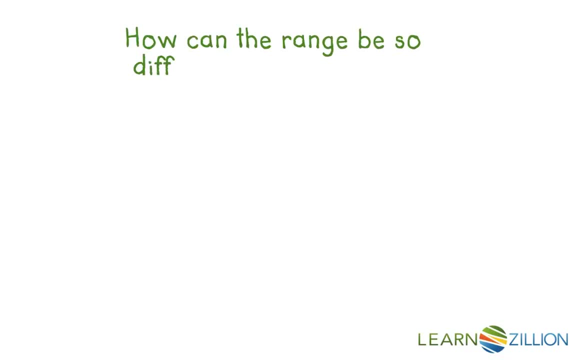 How can the range be so different from other statistical measures? In this case, the median mode and mean are all around 65, but the range is only 8.. How did that happen? In this lesson, you will learn how to describe the distribution of data by using the range. 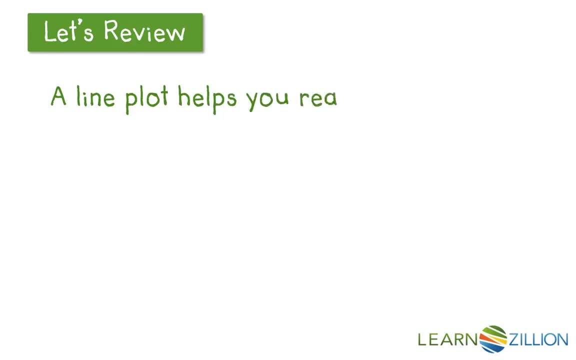 Let's review quickly how to read a line plot. The line plot helps you read data quickly. In this graph, people were asked at what age did you first go on vacation. You can see that the least or smallest answer is 5, meaning 5 years old, and the greatest is 15 years old. 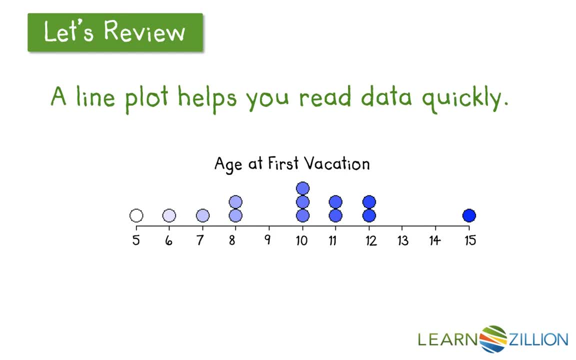 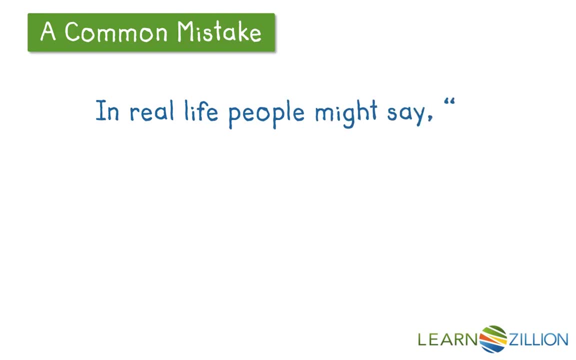 Each dot represents one person's answer, so three people said they were 10 years old on their first vacation In real life. when people use the word range, they will usually state the lowest and highest values, such as the students' age range from 10 to 13.. 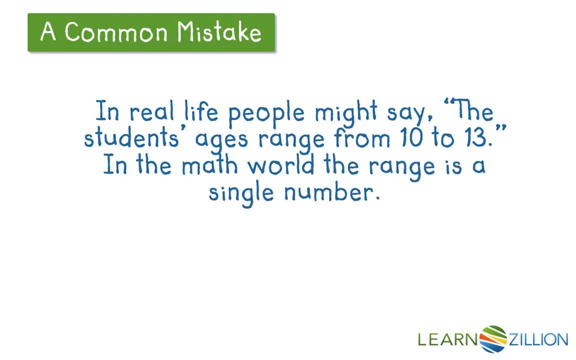 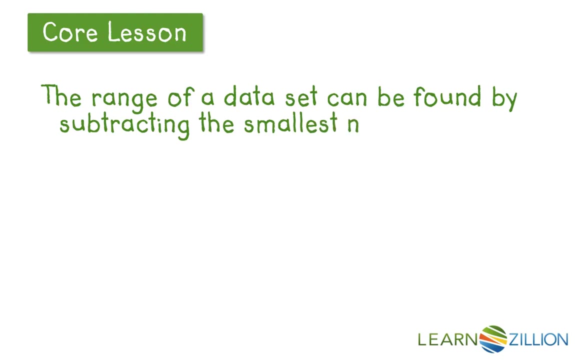 In the math world. range has a similar meaning but a very specific definition. The range is a single number that represents the spread of data. The range of a data set can be found by subtracting the smallest number from the largest number in the set. 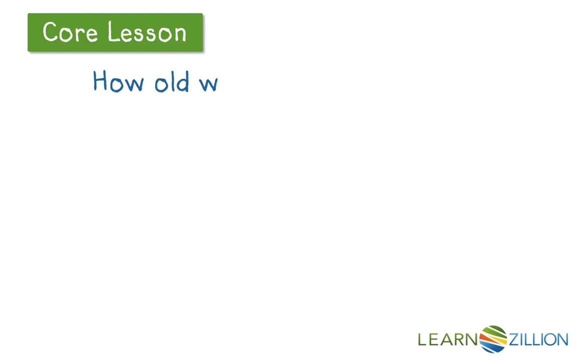 Let's look at some data. The question here is: how old were you when you lost your first tooth? And here is where the response is given. Here is a line plot of that same information And notice how the line plot is very similar to a number line. 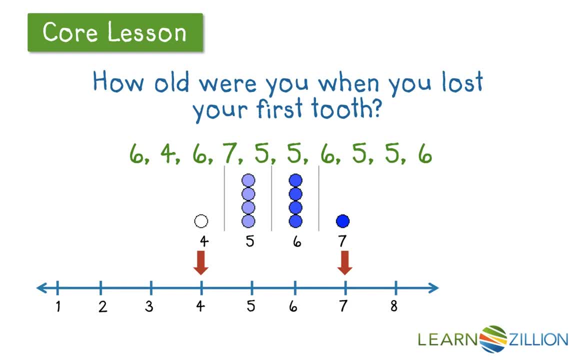 You can easily see the least and greatest answers here. So to find the range, we're going to take the greatest answer of 7 and subtract the least, which is 4, to find the answer of 3.. How does this help us describe the data? 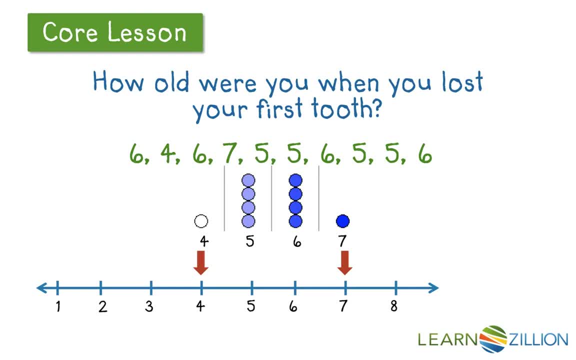 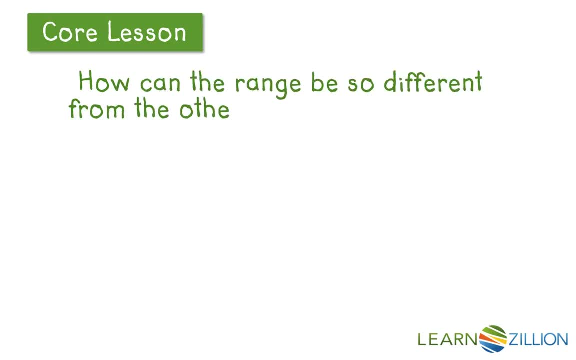 3 is a very low number, which means the answers are all very close together. Let's go back to that original question. How can the range be so different from other statistical measures? When we use the median mode or mean, we're describing the actual data given. 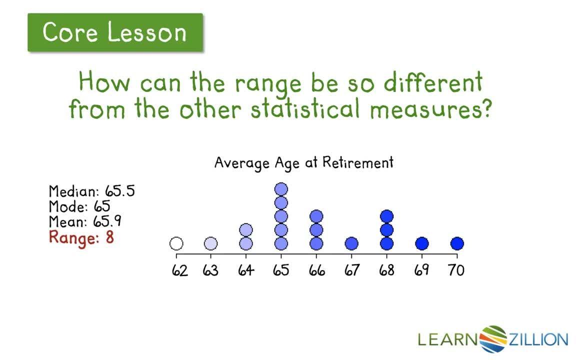 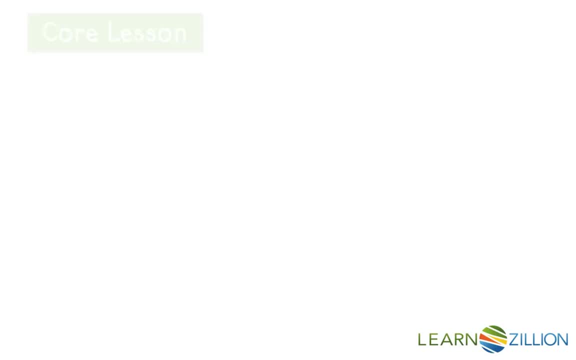 But the range measures the spread of data or how far apart they are. Since the numbers here are close together, the range is small and much smaller than the other measures. Here's another data set. The question is: how many pets do you have? 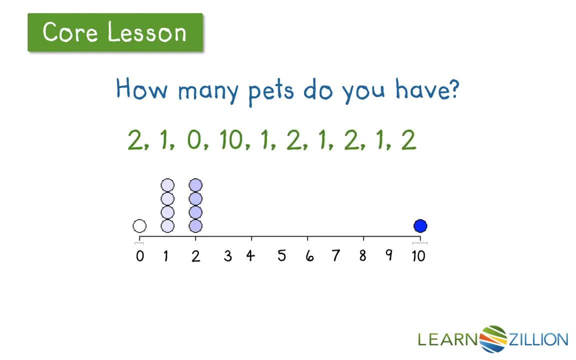 Let's put these numbers now on a line plot. You can see that almost everyone answered 1 or 2 pets, but one person said they have 10 pets. When you have one answer that's much larger or much smaller than most of the answers, that response is called an outlier. 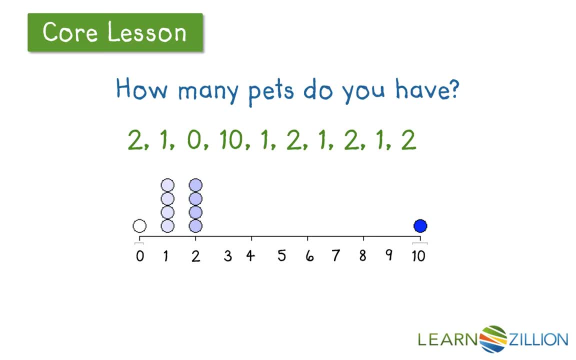 If we include the outlier, the range of this data is 10.. Is a spread of 10 a good way to describe this data? Sometimes mathematicians will leave the answer blank. They will leave the outlier out and recalculate Without the 10, the range would be 2.. 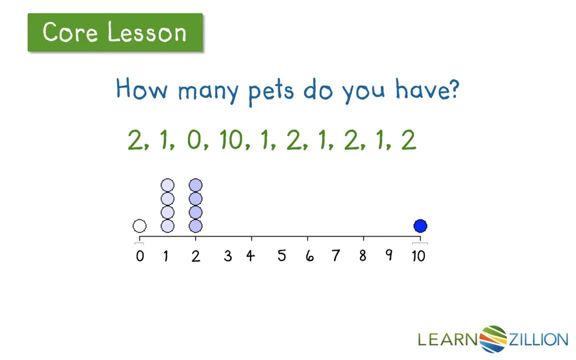 Is the range of 2 a better description of the data. Outliers have a huge effect on the range and the spread. Imagine you're in your classroom and you are asked: how tall are the people in this room in inches? You start to measure the other sixth graders in the room and all of a sudden LeBron James walks into the room. 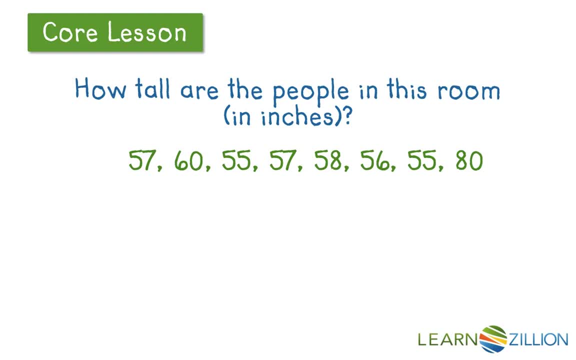 Wow, Look how much taller he is than everyone else. How does this change the spread of the data? If we include LeBron James, the range is 25 inches. That's more than 2 feet and it's a huge spread. LeBron James is an outlier because his height is so different from the rest of the people in the room. 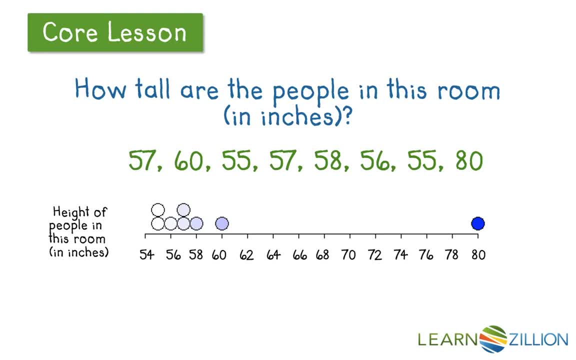 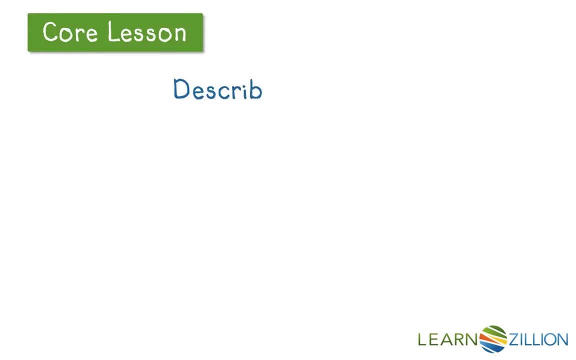 Without the outlier, the range is 5 inches, which is a much smaller spread and indicates that the sixth graders have a very similar height. Sometimes the numbers used in the data set are much larger. In this line plot of house numbers on Lake Avenue, the largest number is 960, and the smallest number is 15.. 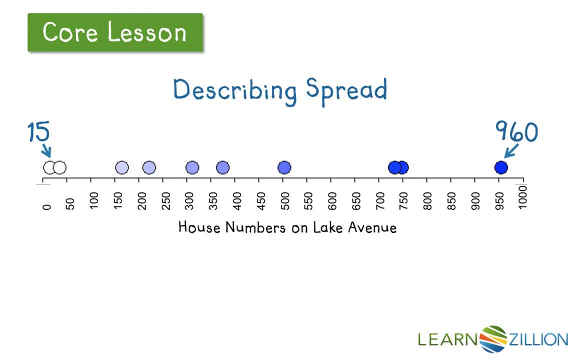 What is the spread of this data? The range is 945, which is a very large range and includes the numbers that are very far apart on the line plot. Compare that to this group with the range of 3.. The range of 3 indicates that the data are very close together and has little spread.